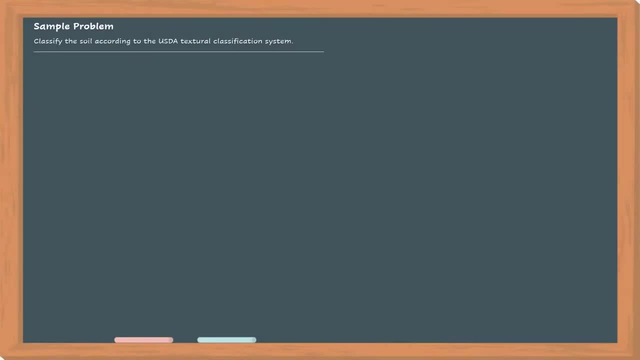 Classify the soil according to the US Department of Agriculture textural classification system. So this is the given information We have: percent of gravel is 12, percent of sand is 25,, percent of seal: 32, percent of clay is equal to 31.. So when we have a USDA textural classification problem, 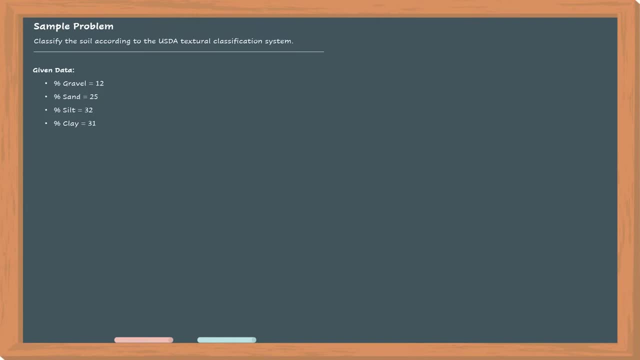 so we have to have the USDA classification chart as triangular in shape, But before that we have to compute first for the modified percent of sand, silt and clay. Why do we need to modify? Because, again, the USDA textural classification. 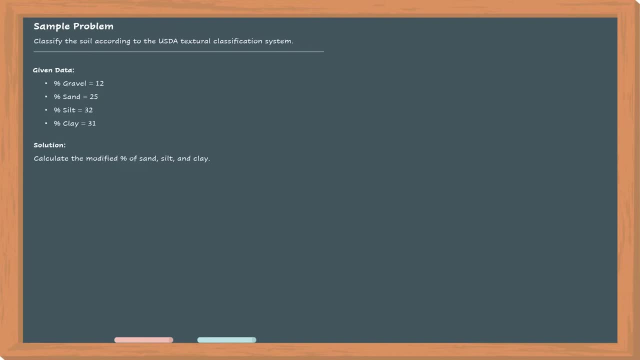 is basing only on the percent of sand, silt and clay, wala siyang gravel. so since meron tayong portion ng gravel, so we have to modify the percent of sand, silt and clay. kumbaga i distribute natin yung percentage of gravel doon sa sand, silt and 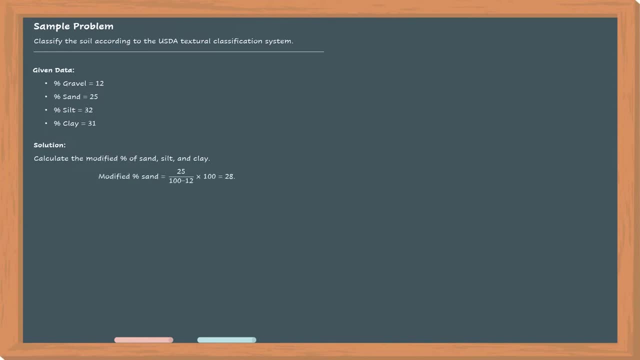 clay. so the modified percent of sand is equal to percent of sand divided by 100 percent minus percent of gravel times 100 is equal to 28.4 percent. and then modified percent of silt is 32 over 100 minus 12 times 100 is 36.4. and then modified percent of clay is equal to 35.2 percent. 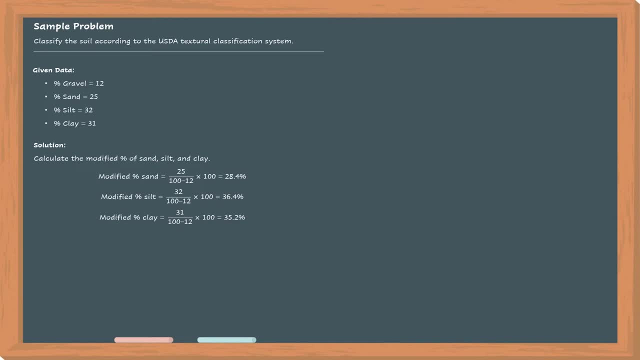 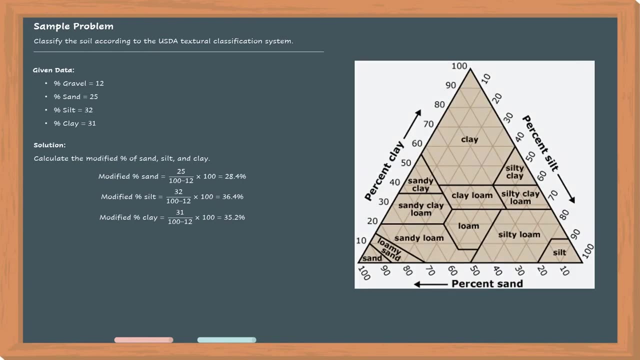 so with these three modified percentages of sand, silt and clay, we can now plot this in the textural classification chart. okay, so let's start with percent of sand. so percent of sand: 20, 28.4 percent. so positive is going to the left. so that means 28 percent is somewhere here. 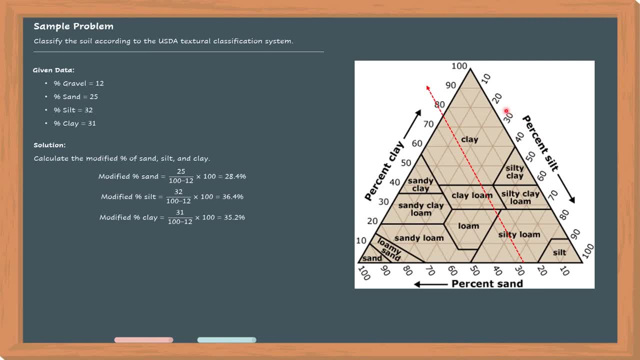 and then percent of silt is 36.4 percent. so let's go to the side of the side of the triangle corresponding to the percent of silt: positive is going down, so let's plot 36.4 somewhere here, okay. and then, um, percent of clay is 35.2. positive is going up, so 35.2 is somewhere here, okay. and then the, the, the.